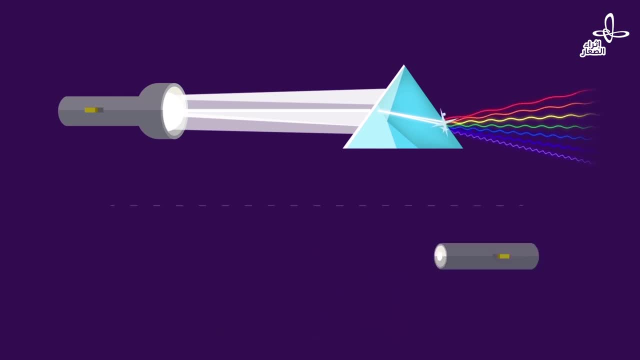 So I bet we can't use it. No, no, it's not weaker. It's beams of light With all the same wavelengths traveling in unison. It's called cohesion. It results in a really strong beam. On the other hand, the light from a flashlight is weaker because the light spreads out as it travels away from its source, the bulb. 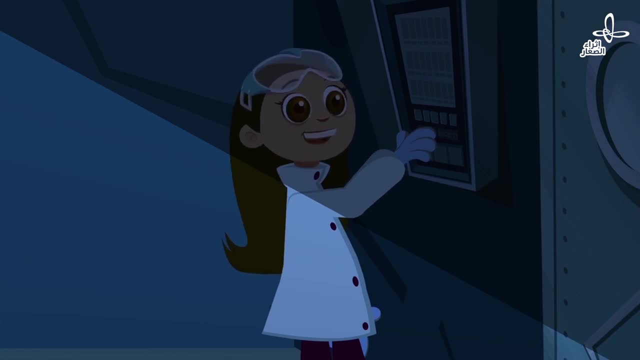 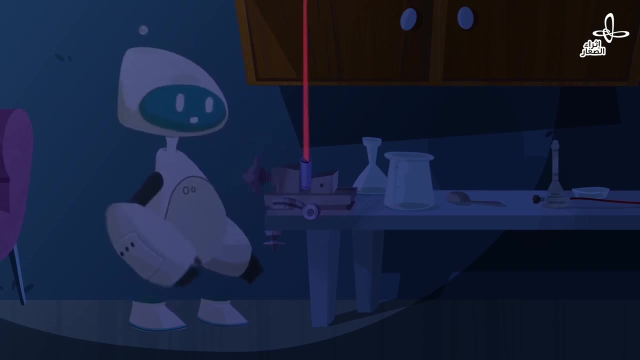 Well, as long as it emits light, we should be able to use it Check. It definitely emits light, Great, But it's stuck, I'm not sure why. Can you fix it? I can't do it. Look at that. 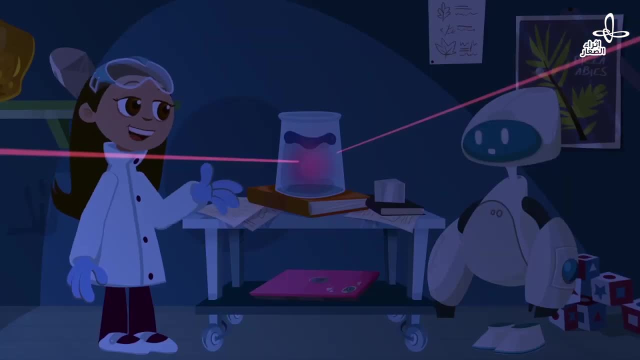 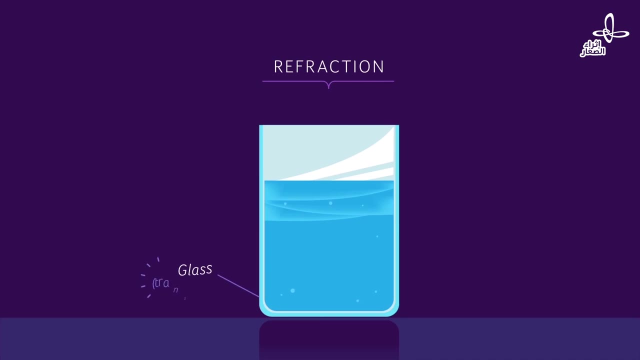 The light has bent slightly through the gel. This must be refraction, Re-whation. It happens when light passes from one transparent material to another transparent material of a different density. Do you get it? I, yeah, not in the least. 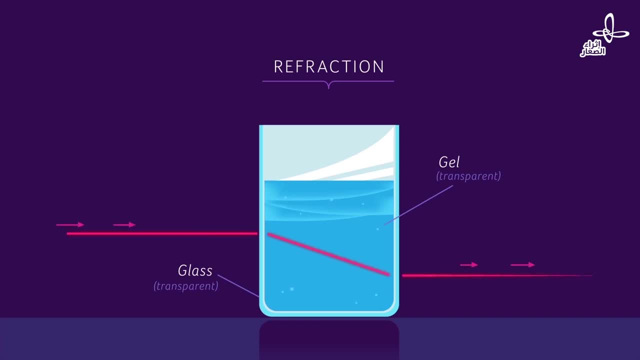 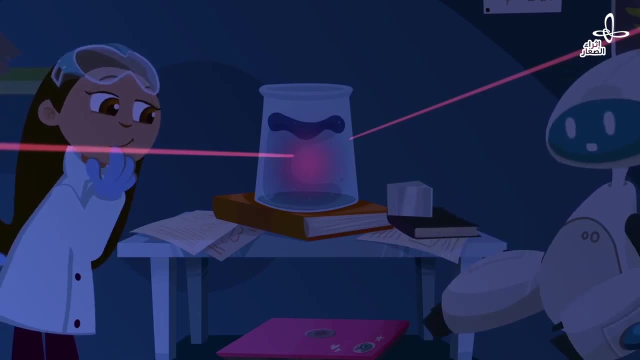 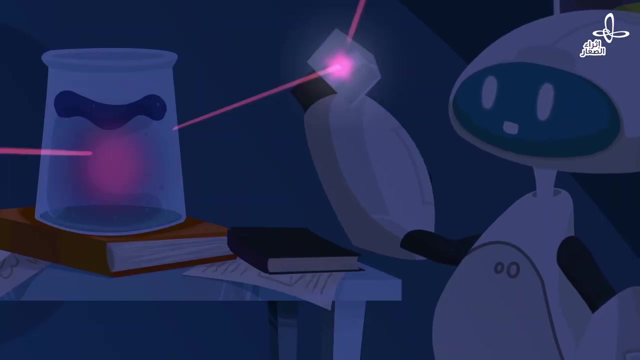 The light is entering at one angle and leaving at another. It's bending. Bend it in your direction, Genius, But how Try other objects in the lab? That's it, Robo. Keep curving it around this way. I bet this black book will help bend the light in your direction. 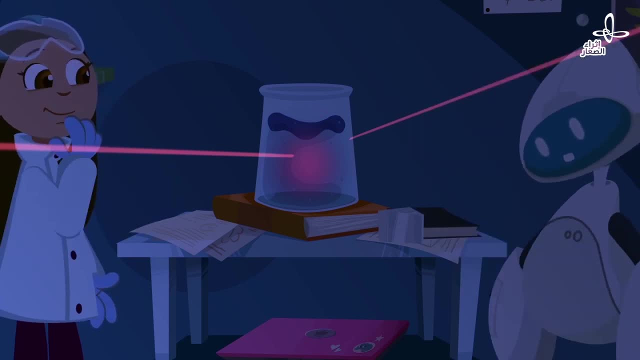 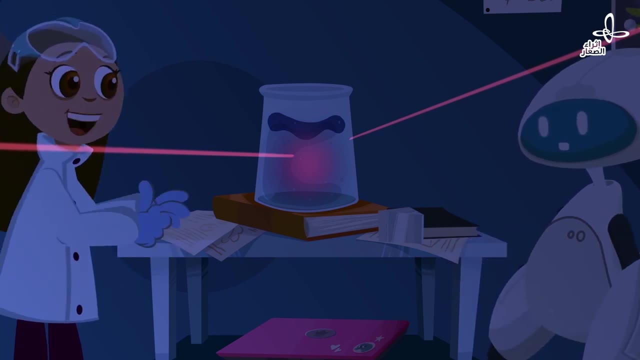 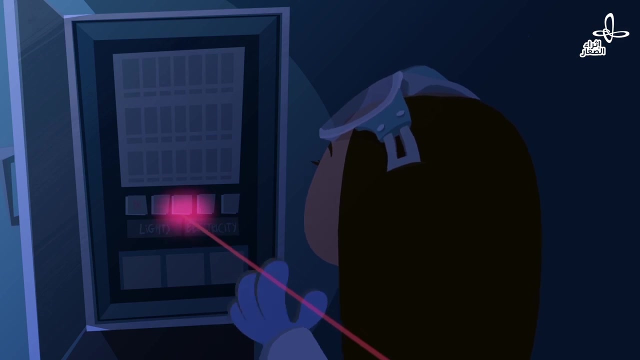 Try everything. we got Nothing. Wait What? Go back to where you were With a book, But it didn't work. No, With your body. Good, Move a little to the left. Good, call Reem Now. move a little bit more to the left. 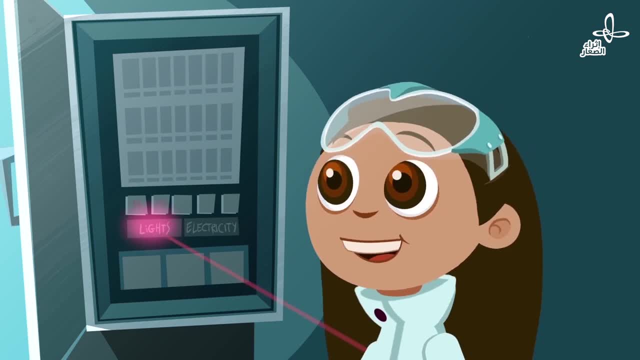 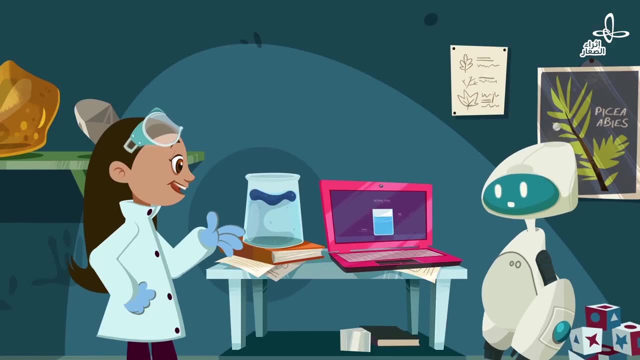 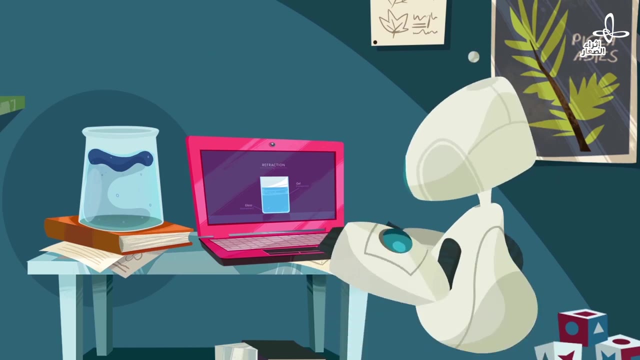 Perfect. I orchestrated a pretty sweet solution. I was going to say that I carried out an amazing solution. Now, what were you saying about reflection and refraction? It looks like we experienced all of the ways that light travels through space: Reflection, refraction and absorption. 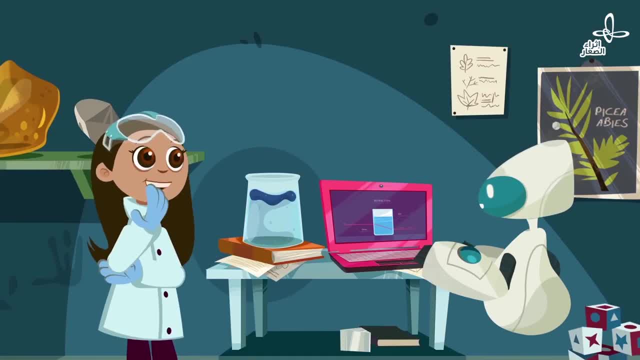 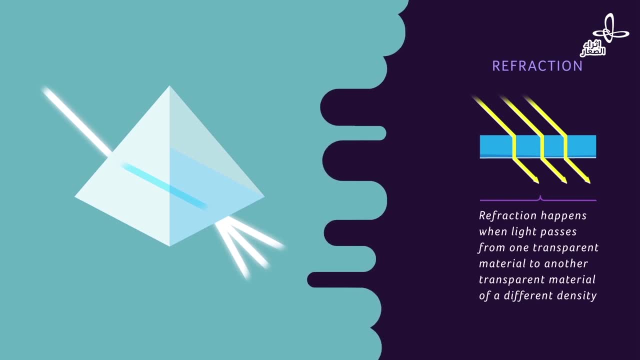 You mean all the ways that light doesn't travel through space. We were in the dark. No, I mean the laser light. When light bent through the clear gel and glass, that was refraction, And then When it bounced off of your opaque, smooth metal body, it was reflection.